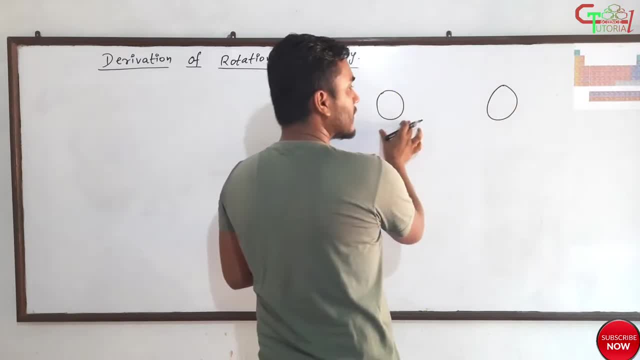 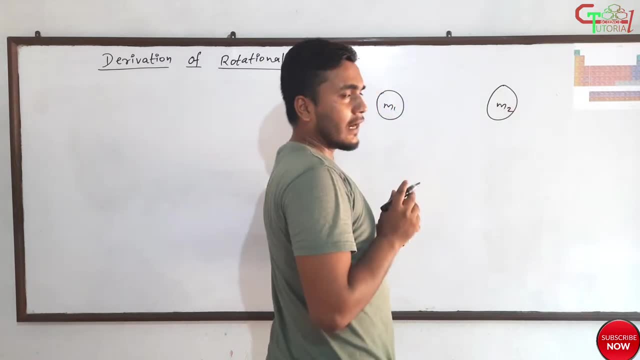 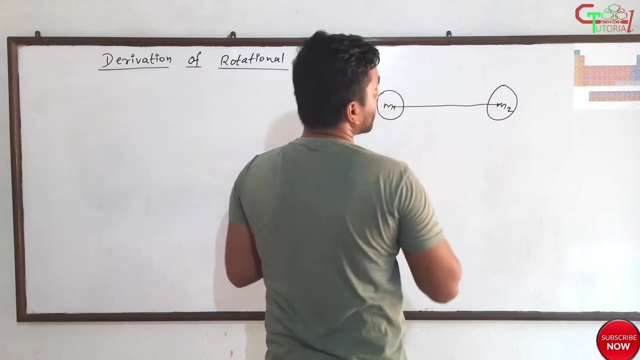 This is a diatomic molecule. This is first atom. This is another atom. Let's consider their masses to be M1 and M2.. And we know that there will be certain sorry, this is the bond. Let's consider: this is the bond. Okay, that is joining their center, And we know that there will be a center. 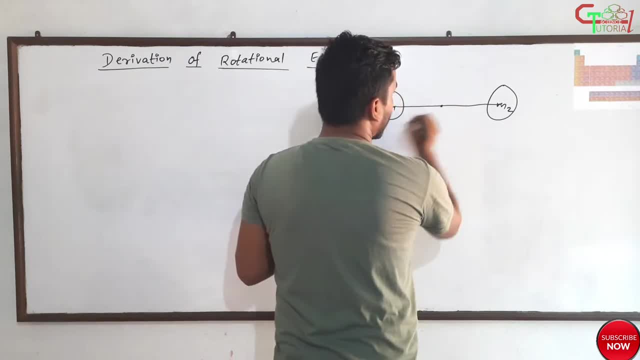 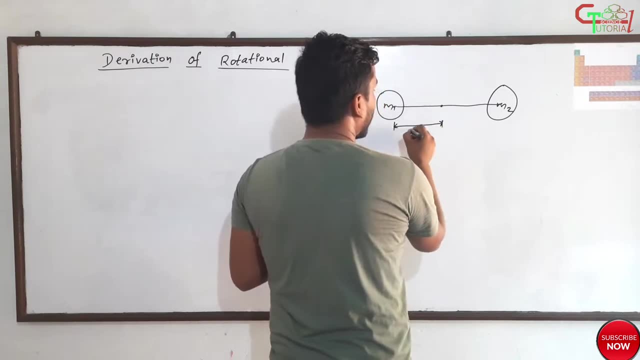 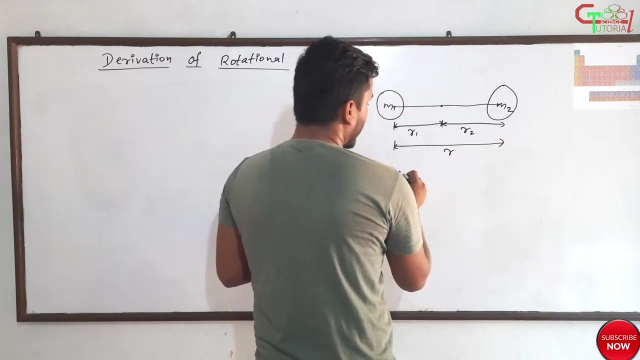 of gravity. Let's consider that center of gravity is here. Then the distance between the center of M1 and this Center of gravity will be R1.. Similarly, the distance between the center of M2 and center of gravity is R2.. And the distance between the two molecules is R. So this is a rigid 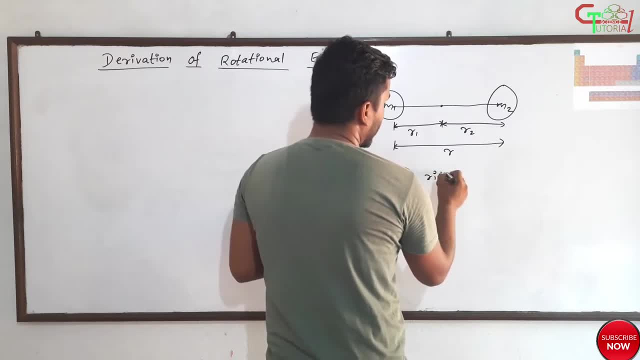 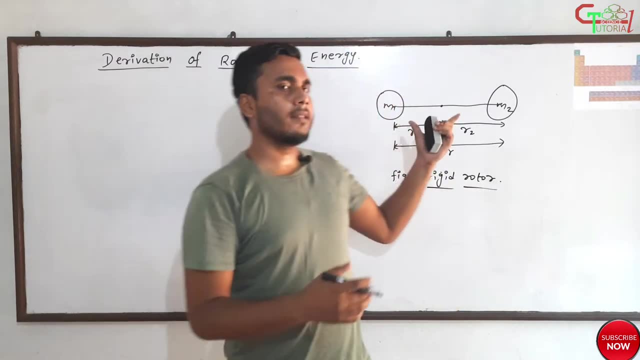 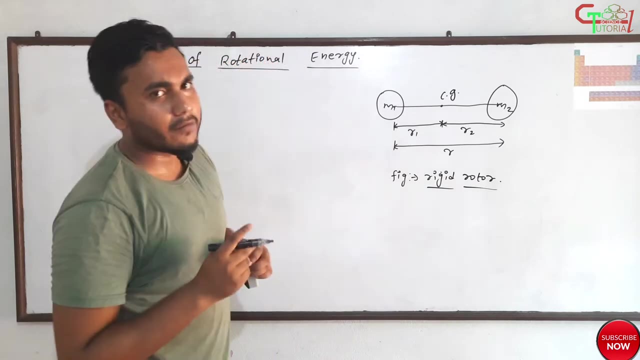 rotor, A rigid rotor. That means we are considering a condition in which they cannot rotate. Okay, Their bond length is fixed, And this is that condition. Now, this is called center of gravity. We already know that At center of gravity, one of the condition is satisfied. Let me 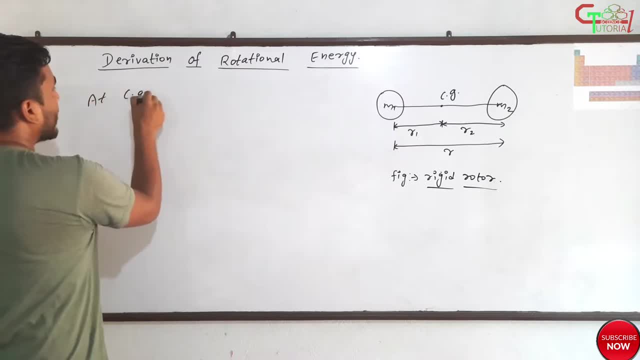 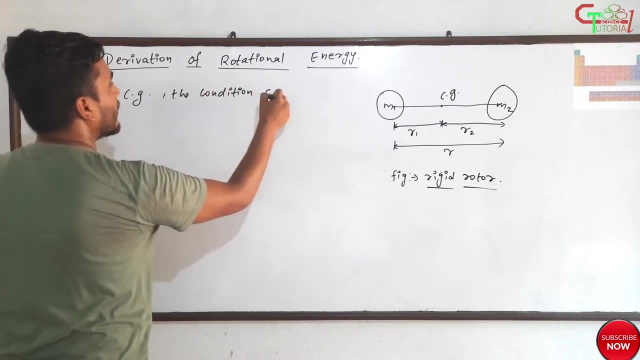 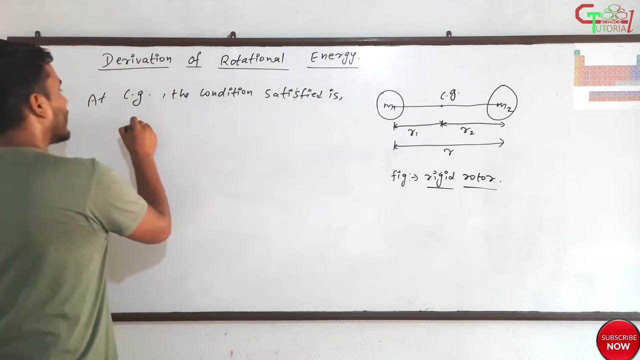 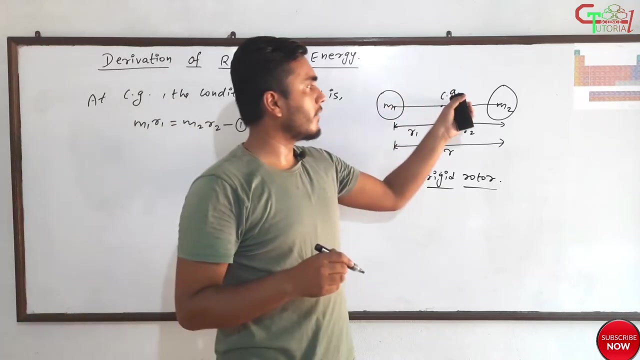 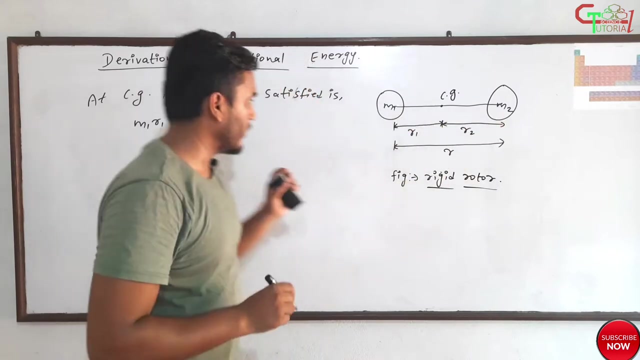 write that, Okay, At center of gravity, the condition, the condition satisfied, satisfied is. the condition satisfied is M1, R1 will be equal to M2- R2.. At center of, at center of gravity, the product of R1 and M1 will be equal to the product of R2 and M2.. Let's consider: 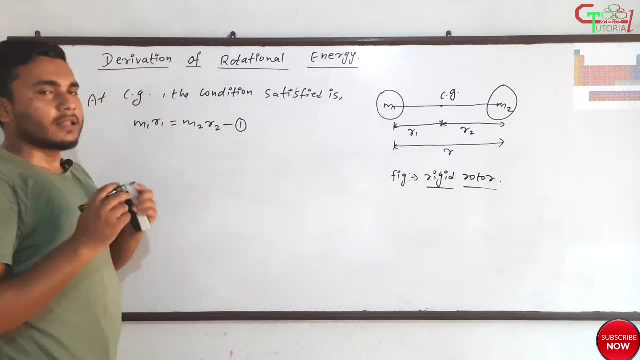 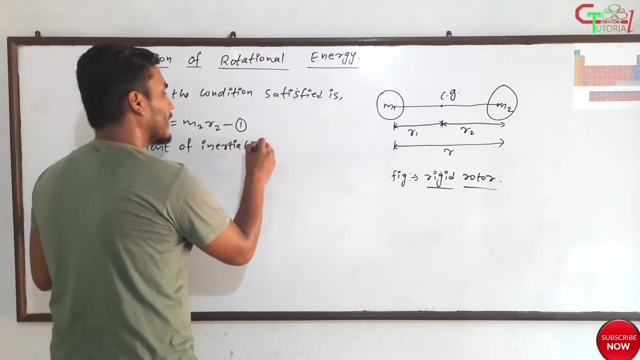 this to be equation number one. Now we know that there will be moment of inertia whenever we talk about rotor right. So the moment of inertia, So the moment of inertia that is denoted by I, Moment of inertia is denoted by I of the 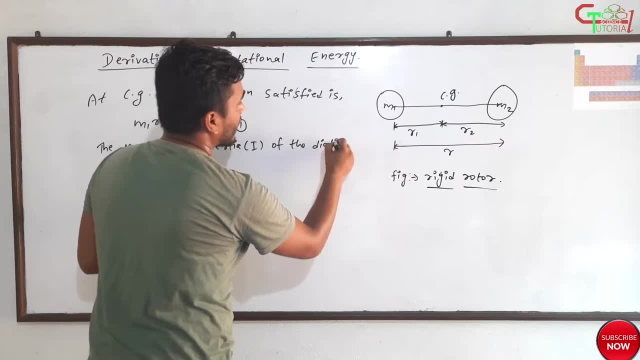 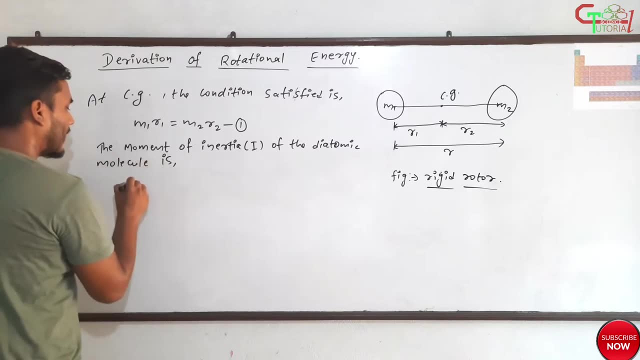 of the diatomic, of the diatomic molecule is molecule, is I will be equal to how much M1 R1 square plus M2 R2 square. So this is the value for the moment of inertia of the diatomic molecule. If it was monoatomic, it would only be: I is equal to M1 R1 square. Now it is diatomic. 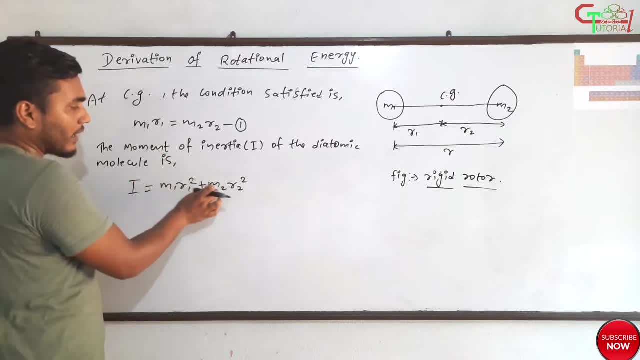 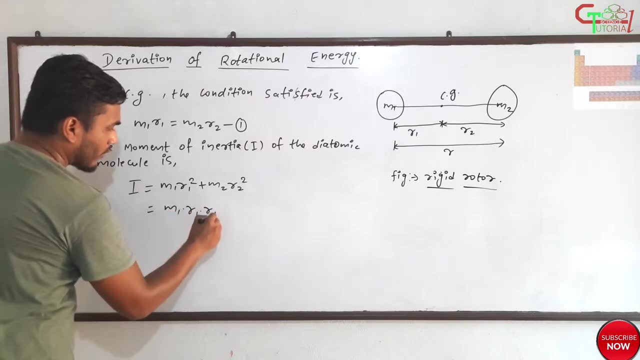 So we need to add M1 and one: M1- R1 square and M2- R2 square. Now can we write this like this: M1 into R1 into R1 plus M2 into R2 into R2.. Obviously, we can write this right Now. let's use equation number. 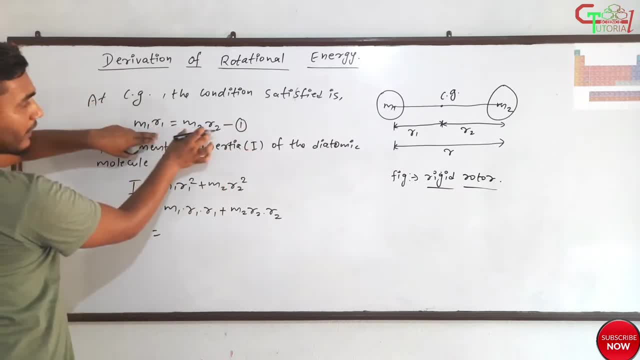 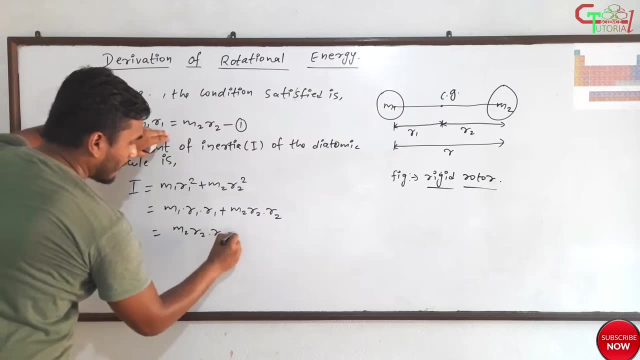 one over here. That means in place of M1 R1, we can write M2 R2.. Here there is M1 R1.. So let's write M2 R2 over here. M2 R2 into R1 plus. 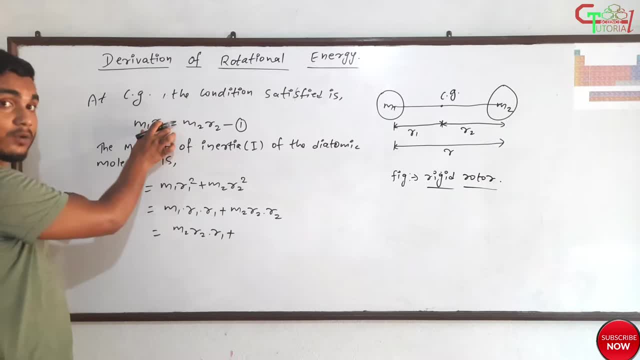 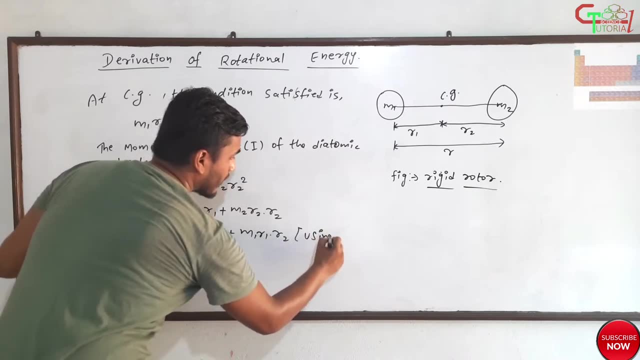 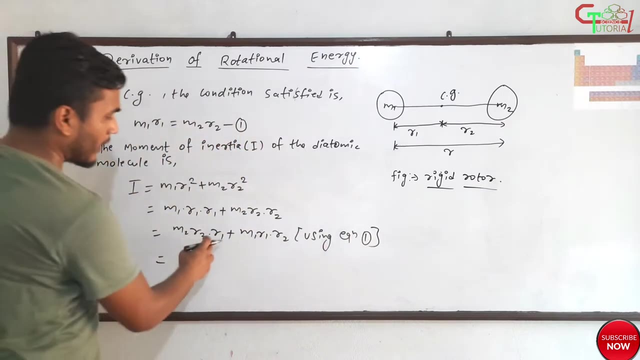 here, in place of M2- R2, we can write M1- R1,. right, So let's write M1 R1 into R2.. We are using- we are using equation number one over here. Okay, So we get. let's take common R1- R2, R1- R2 can be. 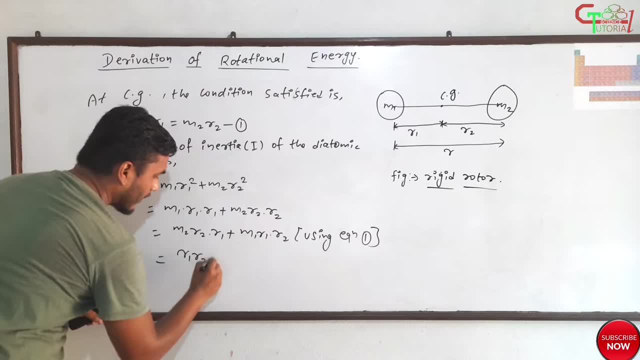 taken as the common. So let's take them as the common: R1, R2.. We get M1 plus M2.. So this is how much we get If we solve this. we get M1 plus M2.. So this is how much we get. So this is how much. 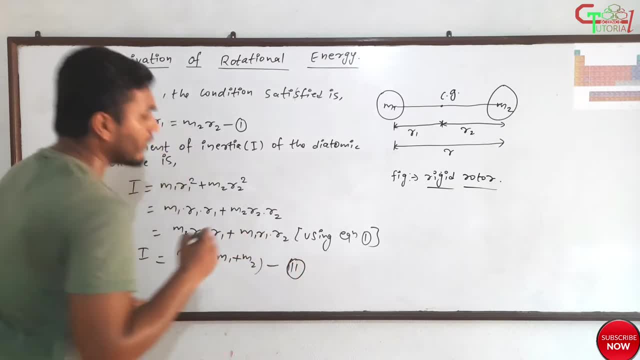 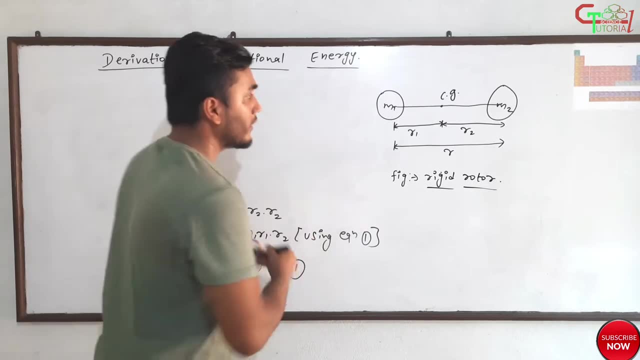 we get If we solve this equation, and let's consider this to be equation number two. Now to do further, let me erase this part. Now. from the figure we can write that if we add R1 and R2,, 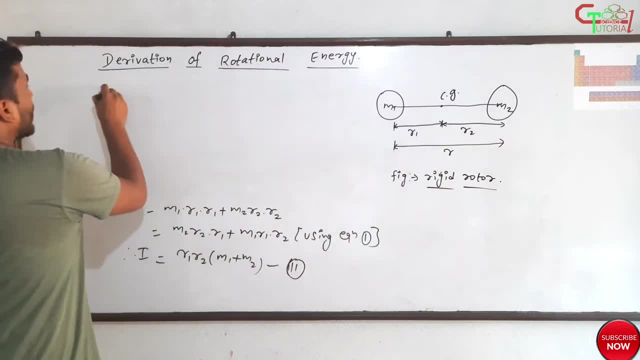 how much will we get? We will definitely get the value of R. So from figure from figure, we can write: R1 plus R2 will be equal to R. Now, from this, let's find the value of R2.. So 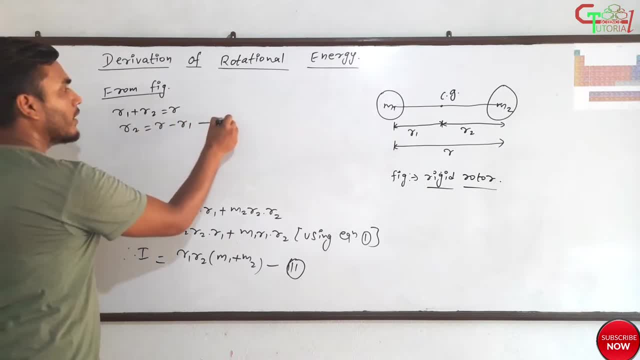 R2 will be equal to R2.. So R2 will be equal to R2.. So R2 will be equal to R2.. So R2 will be R minus R1.. Let's consider this to be equation number three. We can consider it right Now. 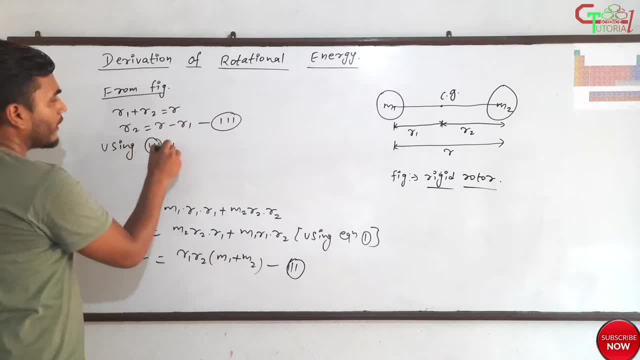 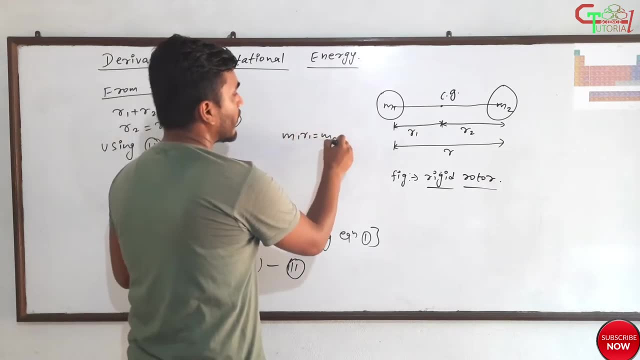 using equation number three in equation number one. What was equation number one? I have already read that, but it is M1. R1 is equal to M2, R2, right? So here, in place of R2, let's write the. 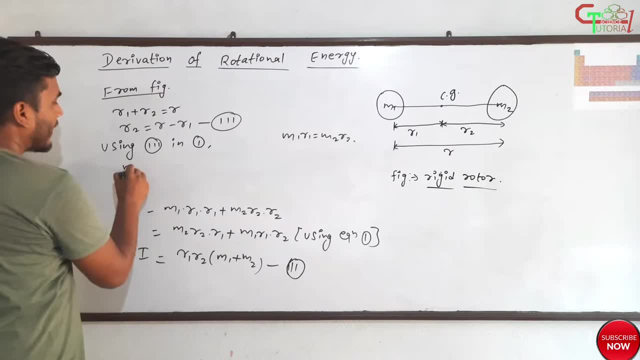 value of R2 from here. okay, So it will be M1 R1, equal to M2, into in place of R2.. What do we need to write? M1 R1 is equal to M2- R2.. So let's write the value of R2 from here. okay, So it will be. 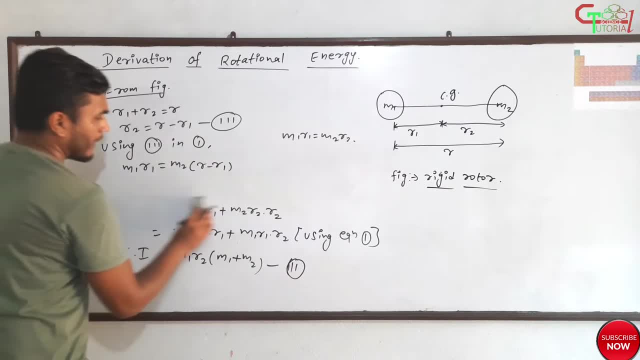 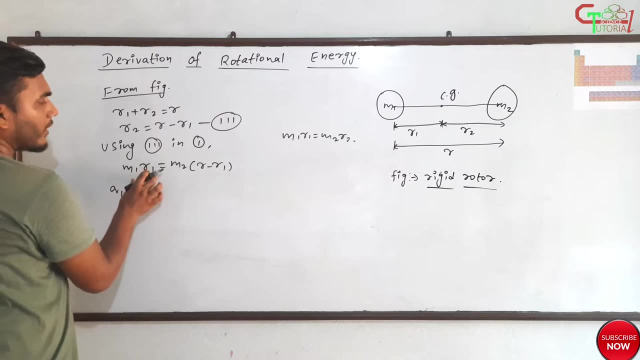 R minus R1, right, Let me erase this part. okay, Now let's solve it from here. We need to find the value of R1, okay, So it will be M1 R1 equal to M2 R minus M2 R1.. Let's take this value to this. 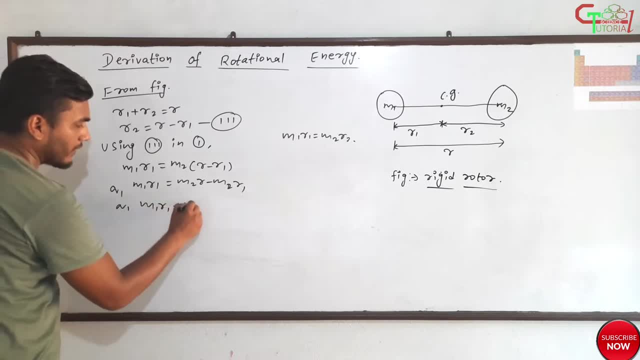 side, Then its sign will. what Change? obviously, So it will be this much. So therefore, it will be: R1 will be equal to. if we take R1 common, it will be M1 plus M2.. If we 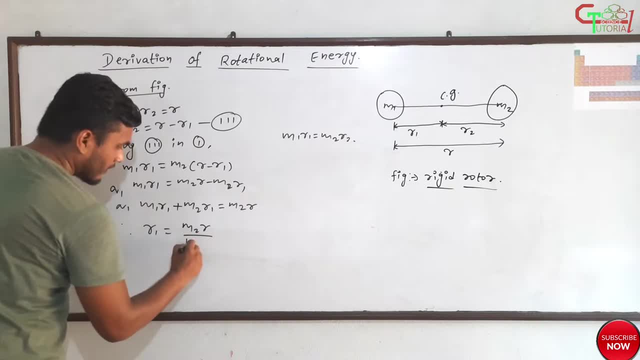 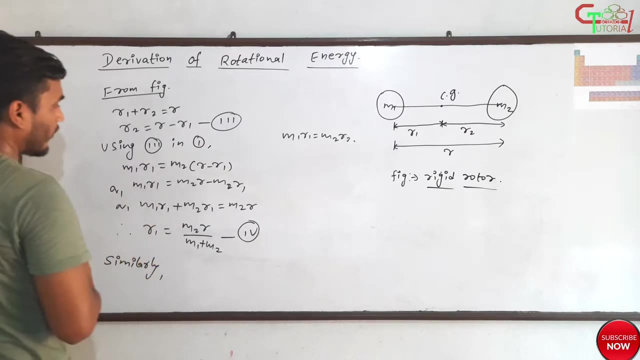 take it to other side. it will directly be this much. right, It will be this much. Let's consider this to be question number four. Similarly, if we found the value of R1 over here, then it would have been R2- R1.. So it will be R2- R2.. So it will be R2- R2.. So it will be R2- R2.. So it will be. 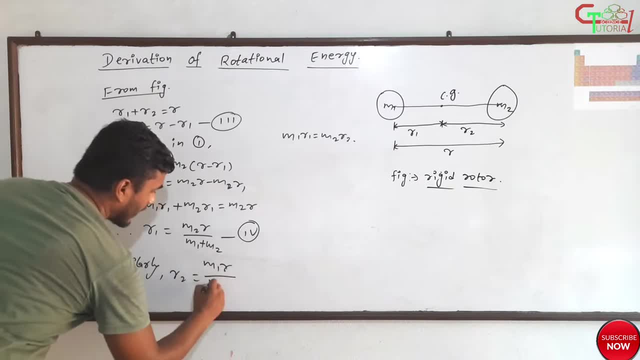 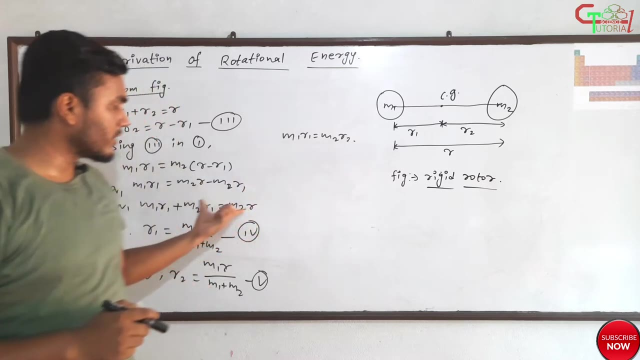 equal to M1, R by M1 plus M2.. You can easily do this by finding the value of R1 over here. Take R2 to other side and put the value of R1 here. Then if you find the value of R2, just like this: 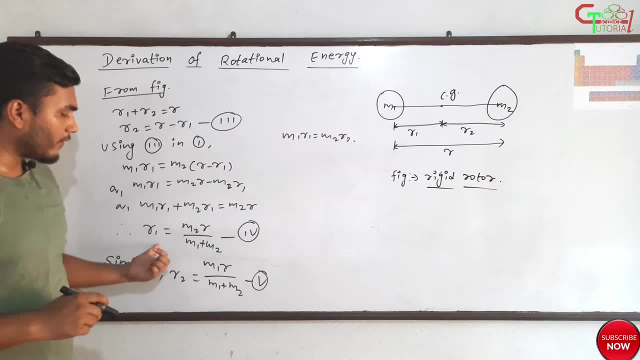 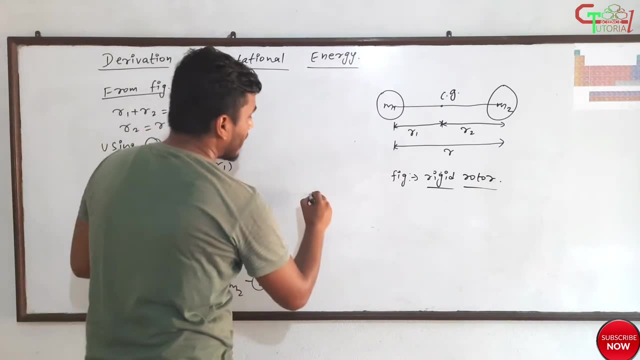 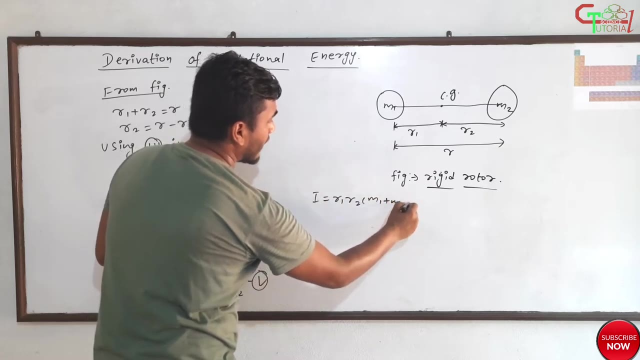 you would get this much. So we now found the value of R1 and R2.. Now we need to put these values in equation number two. What was equation number two? Equation number two was: I is equal to R1 into R2, M1 plus M2, right, This is equation number two. Now let's put: 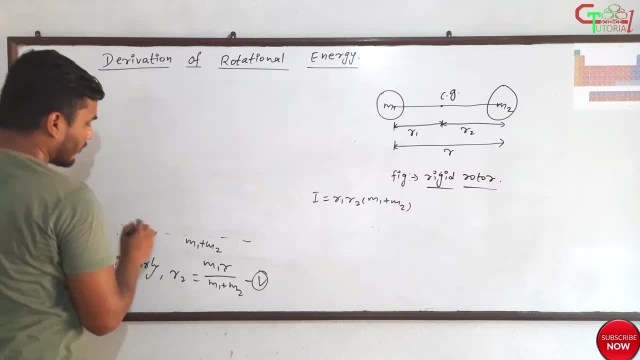 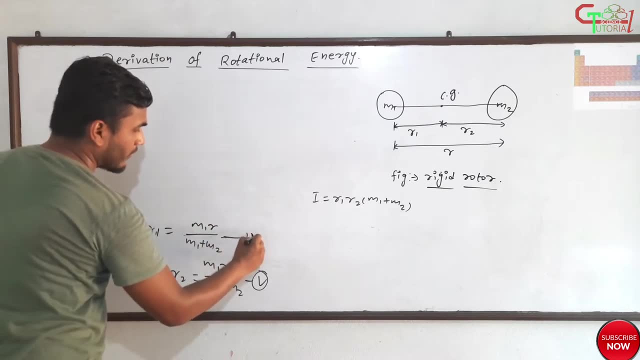 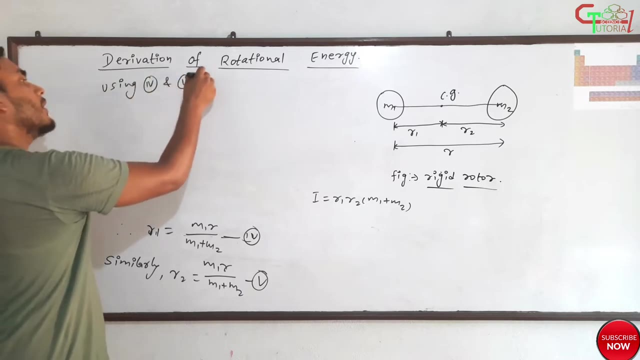 these values, the values of R1 and R2 in equation number two. okay, This was equation number four. Now using four and five in two. So, using these two values, this is R1, actually The. using these two values in this equation, what will we get? I is equal to in place. 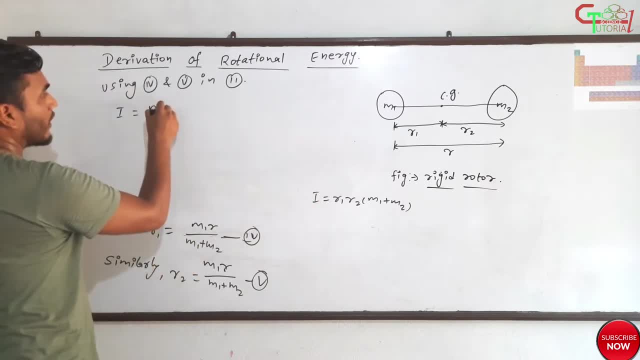 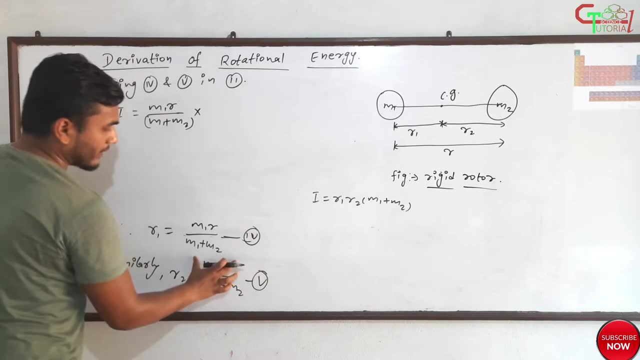 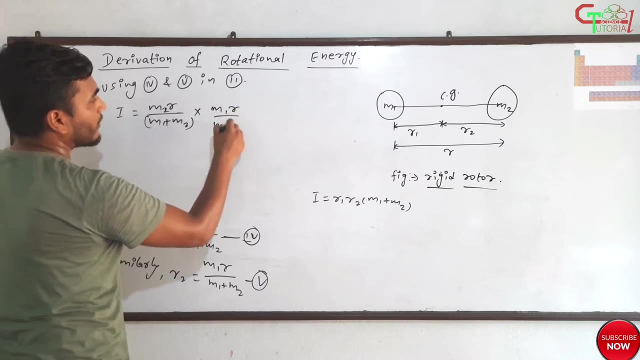 of R1, we need to write this value, that is, M1 R by M1 plus M2, into in place of R2,. let's write this value- Sorry, here it should be two- So M1 R by M1 plus M2 into how much M1 plus M2.. 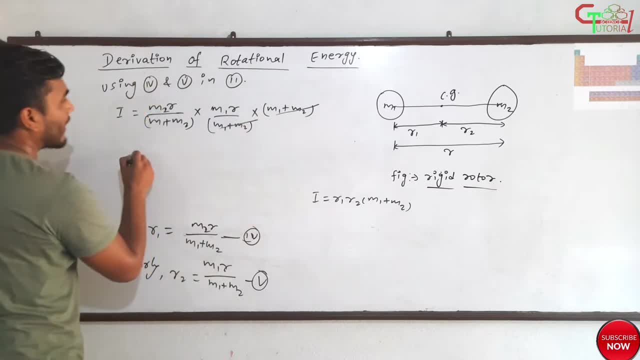 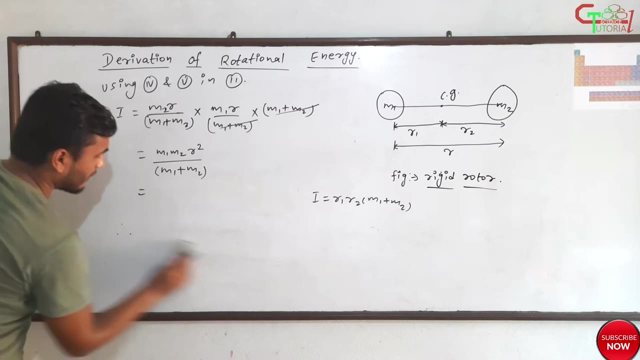 M1 plus M2, right. So we can cancel these values and we just need to multiply M1 into M2 will be M1, M2.. R into R will be R2. by it will be M1 plus M2, right. Now you can see over here. let me read. 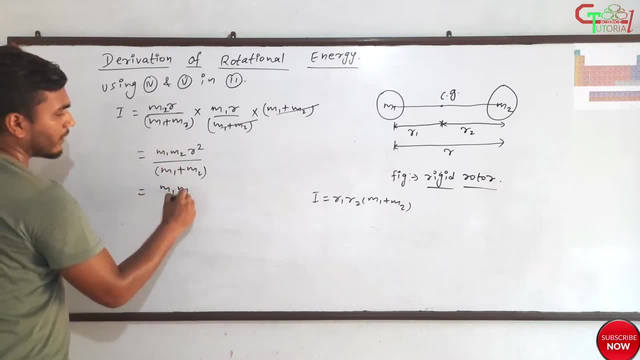 this part You can see over here. let's just write this part together: M1 plus M2 into R2.. Now this can be represented by mu. Mu means combined mass right Or reduced mass. So I will be equal to this much. Let's consider this to be question number. 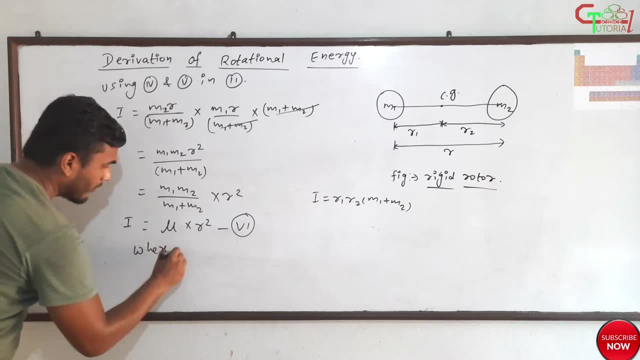 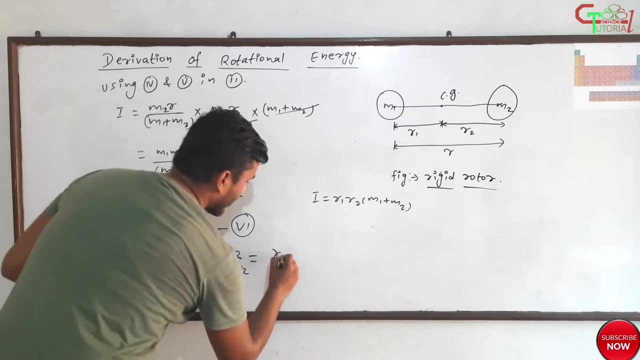 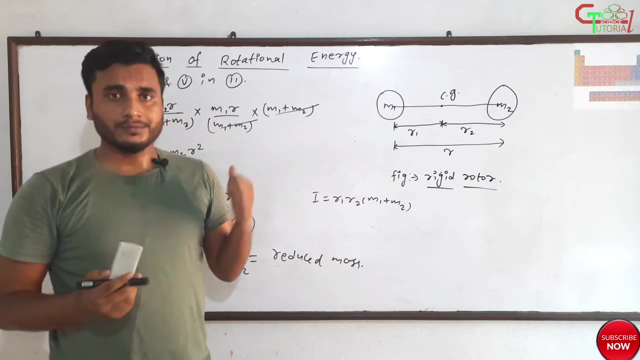 C 6, where mu is equal to M1, M2 by M1 plus M2, which is the reduced mass. Now for further derivation. let me read this portion. Now we need to use the concept of angular momentum. 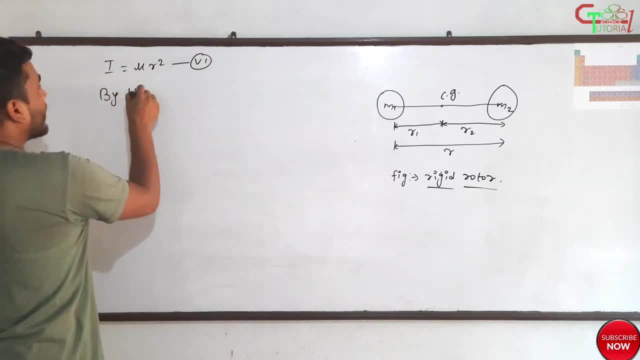 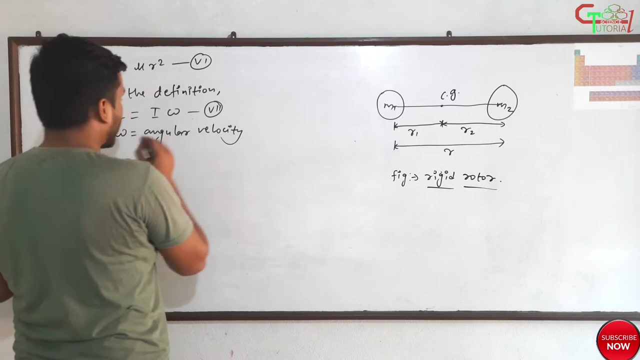 So by the definition, the definition, the angular momentum, the angular momentum, that is L, can be written as I, omega, where this omega is the angular velocity. Angular velocity, This is equation number 7, okay, And this I is the moment of inertia. L means angular momentum, okay, So here L means 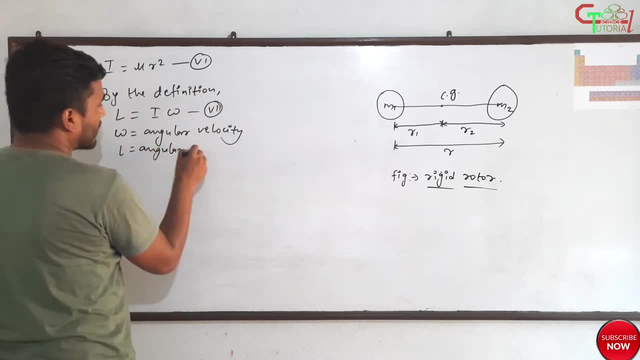 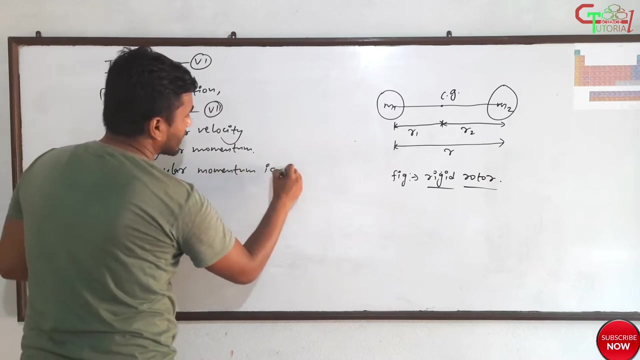 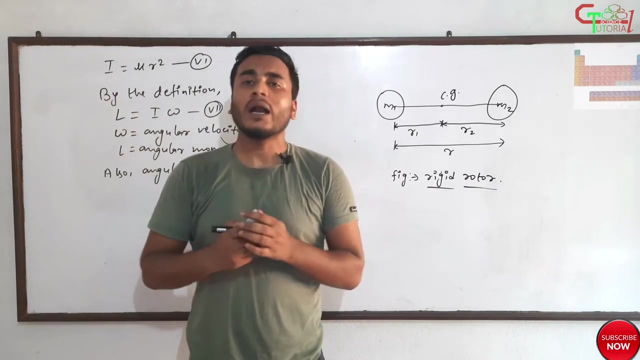 what Angular Angular momentum? Angular momentum Also angular momentum. this is very important point. Angular momentum is quantized, Quantized. Quantized, The meaning of quantized means it depends on the quantum number. okay, It depends on the quantum number. That's why angular momentum is quantized. 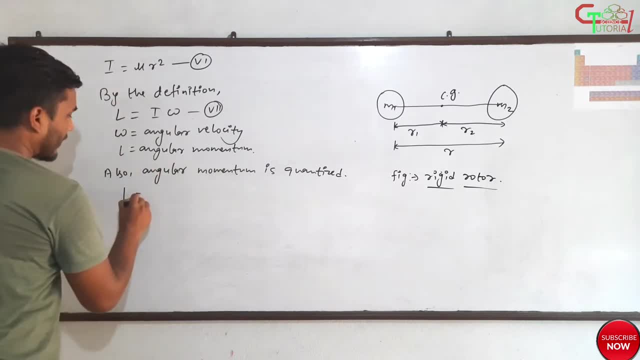 Now its formula. another formula can be given as root under J into J plus 1, into H by 2 pi. This can also be the formula. This is also a formula for angular momentum in terms of quantum numbers. okay, So let's consider it to be equation number 8.. Now the rotating energy. the rotating 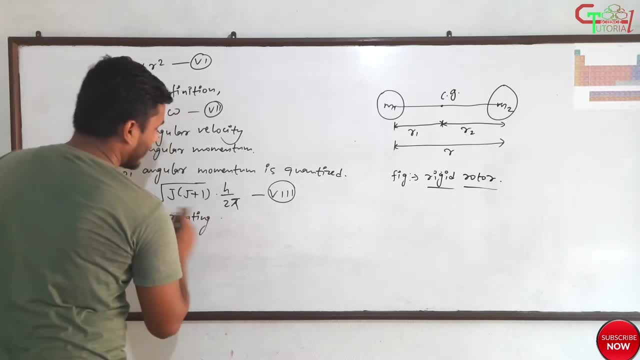 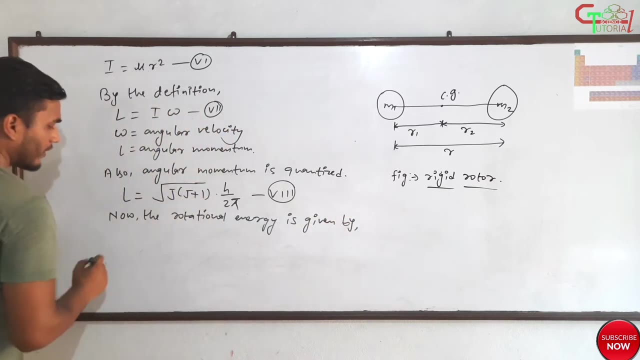 energy or rotational energy. okay, It would be better to write rotational energy. The rotational energy is given by, given by. there is a formula for the rotational energy and that is to be equal to half I, omega square. This is the formula for the rotational energy. Now let's do something. 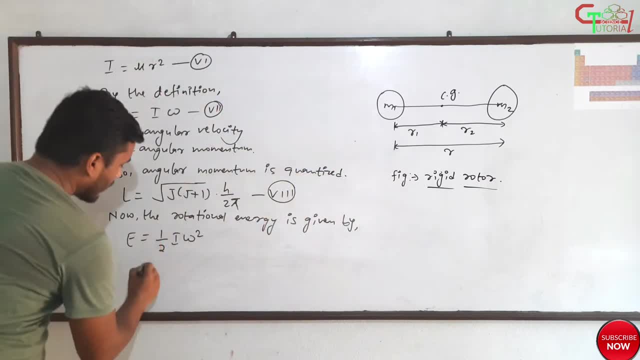 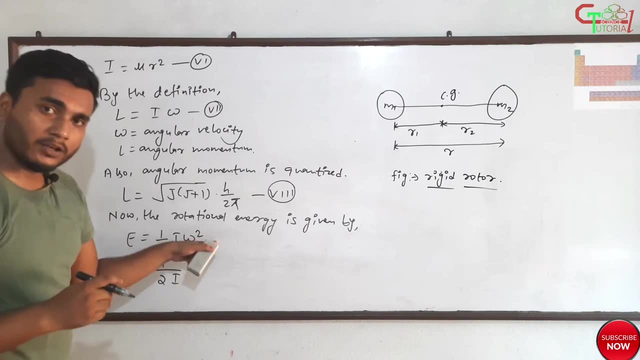 about the rotational energy in terms of constant terms. okay, So we can write like this: 1 by 2 I. If we write I in the denominator, we need to multiply 1 I in the sorry with the numerator. 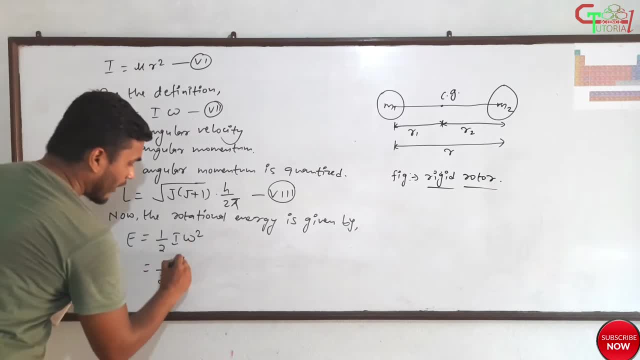 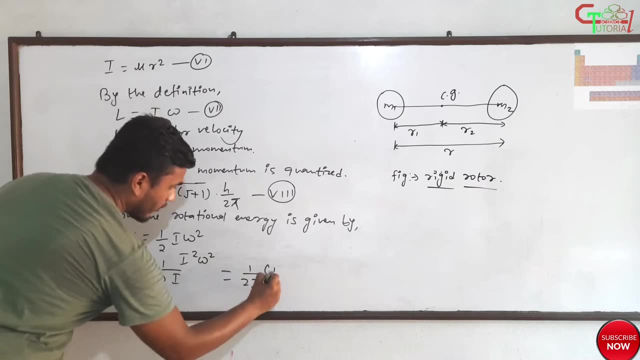 If we multiply there, it will be I into I. So it will be how much I square, omega square, right, So it can be written as 1 by 2: I into I, omega square. Can we write this or not? And in place of 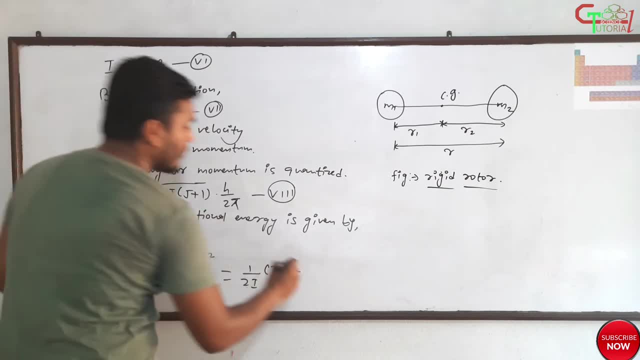 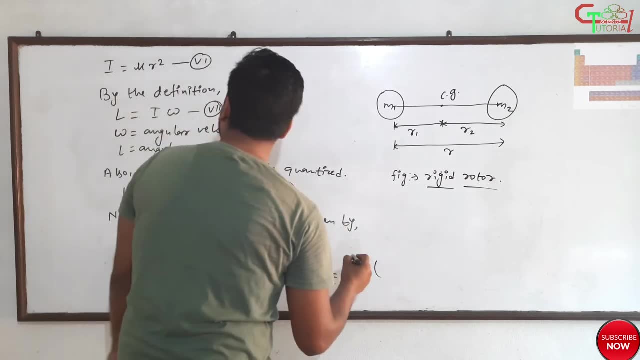 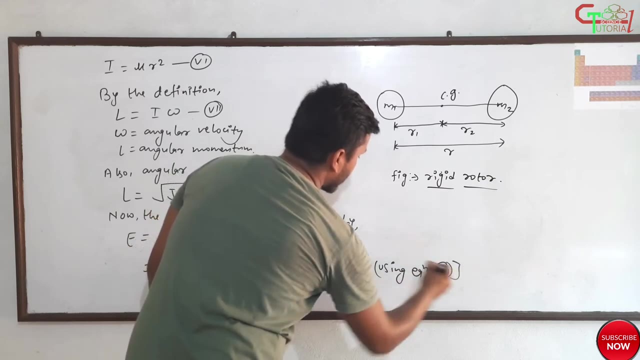 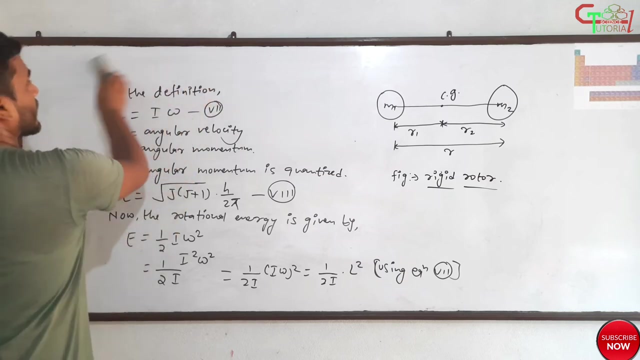 I omega. what can we write? means L, so we can write half 1 by 2i into L square. and this is we get by using equation number. using equation number, how much 7? so we we get this much of the value right. so let's erase this portion. let's erase this portion. 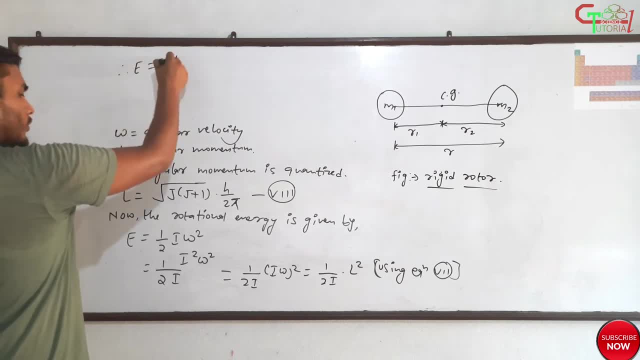 therefore, how much do we get? energy is equal to 1 by 2i. into how much L square but L? we need to find the value of L in terms of quantum number right and it is given here in the equation 8. so using using equation number 8, if we 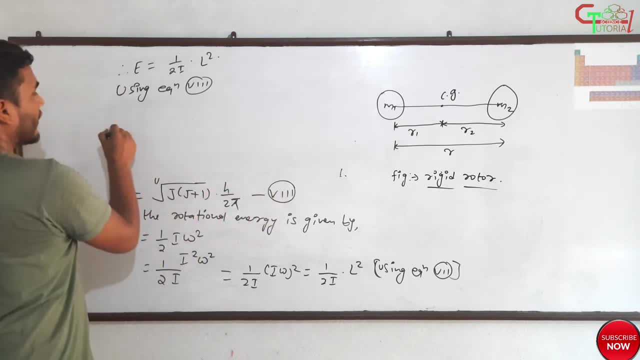 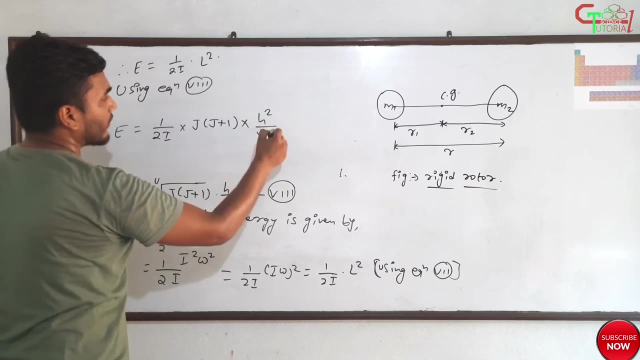 use the equation number 8 over here, then what do we get? E is equal to 1 by 2i into there is square, right. So this root will be cancelled out. So it will be j into j plus 1 into h, square by 4 pi r, 4 pi square. Yes, we will get this much and it will finally be how. 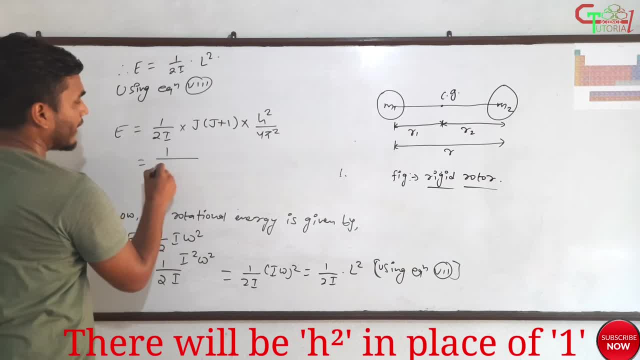 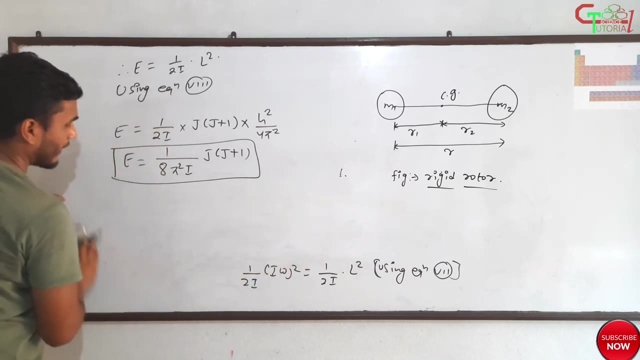 much. If we multiply, then this two fossa will be 8 pi square i into j, j plus 1.. So this is the required value for the energy of rotational energy, or simply rotational energy formula. okay, This is called. this equation is called rotational energy formula. Here we can see: 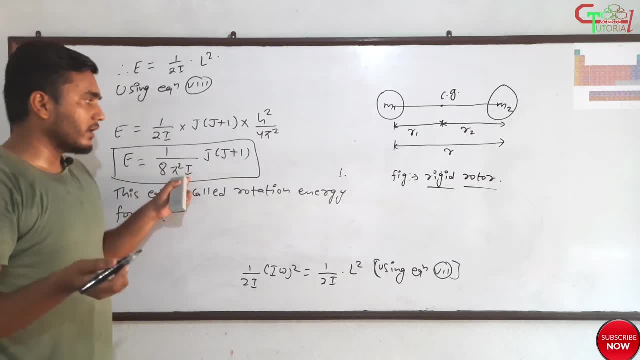 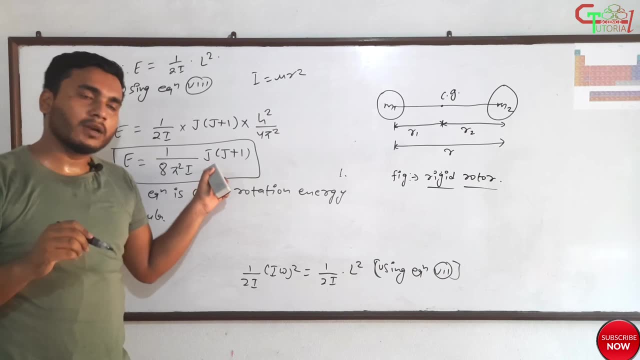 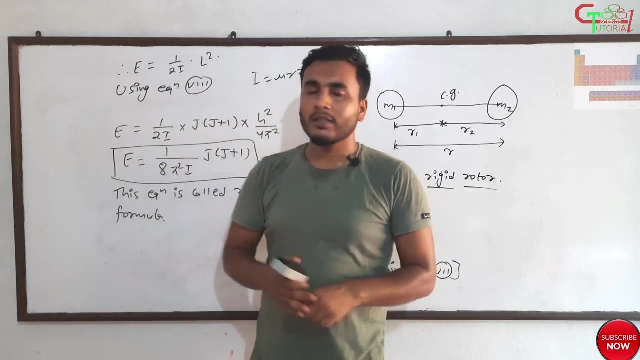 that this i can be calculated mathematically by using the formula: i is equal to mu r square, and this j is the rotational quantum number that we can know and by using which we can find the rotational energy easily. So this is the formula for the rotational energy. 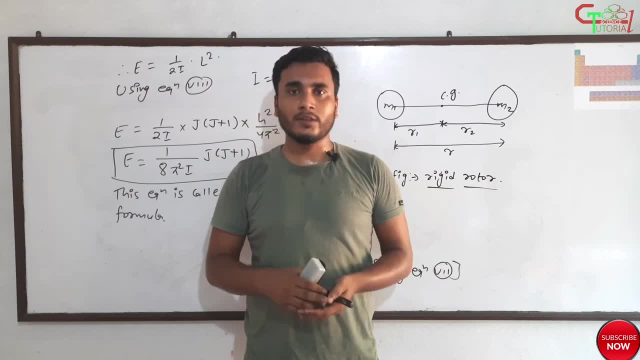 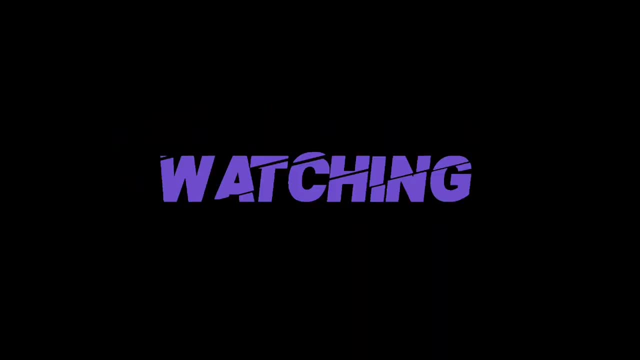 That's all in this video. If you like the video, please share this video as much as you can. Thank you for watching the video. See you in the next video.